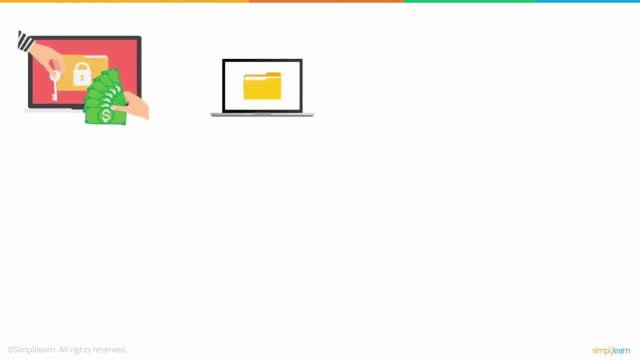 as gateways for a ransomware breach. Ransomware is a type of malware that encrypts personal information and documents. It is a device that causes the hackers to make attacks by smuggling and trading information, while demanding a ransom amount to decrypt them. But how does it decrypt the files? 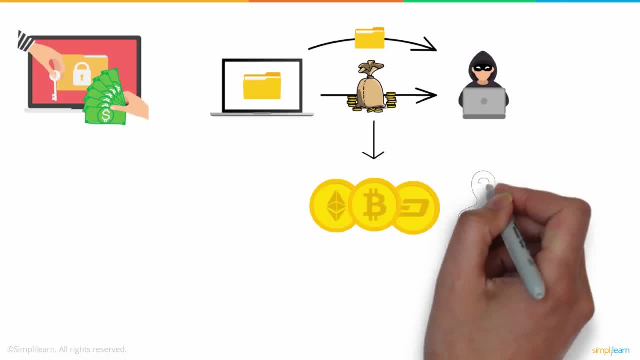 This ransom payment is mainly done using cryptocurrency to ensure anonymity, but can also employ other routes. Ransomware is a device that can be used to decrypt a number of files, but it can also be used to decrypt a number of files Once the files are encrypted or locked behind. 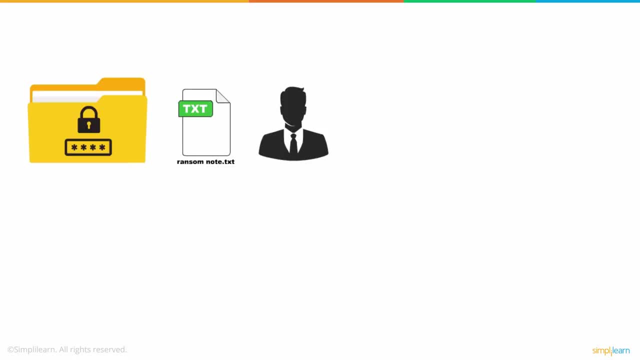 a password. a text file is available to the victim explaining how to make the ransom payment and unlock the files for it, Just like Richard found the Ransom Note text file on his desktop. Even after the money has been paid, there is no guarantee that the hackers 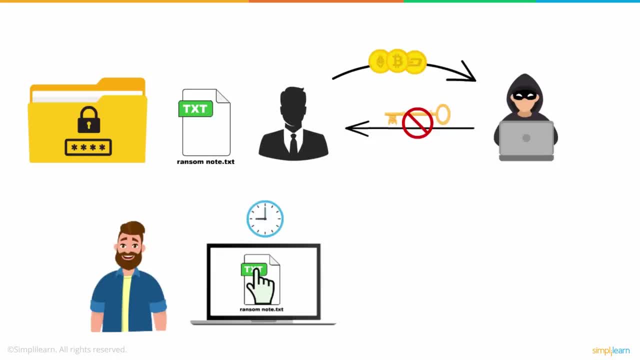 will send the decryption key on this device Or unlock the ransom file on a ransom note. So does it mean that the hackers will send a ransom key to the intéressant ransom note key or unlock the files? But in certain sensitive situations victims make the payment, hoping for the best. 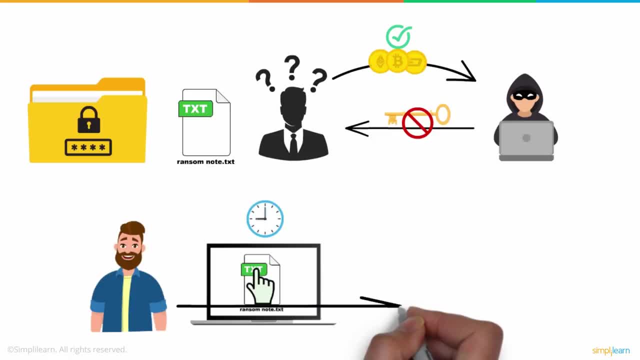 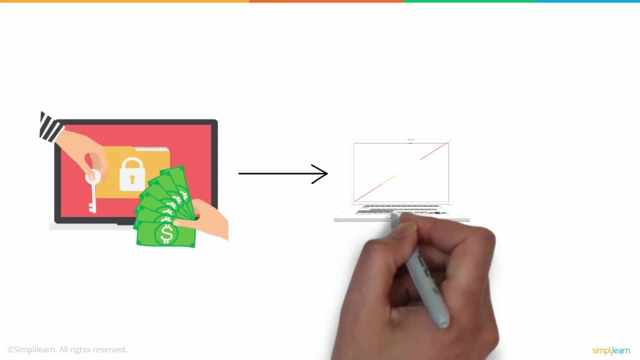 Having never been introduced to ransomware attacks before. this gave Richard an opportunity to learn more about this and he began his research on the topic. The spread of ransomware mostly starts with phishing attacks. To know more about phishing attacks, click the link in the button above. 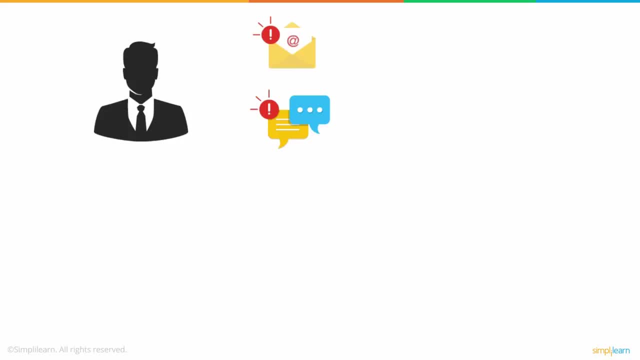 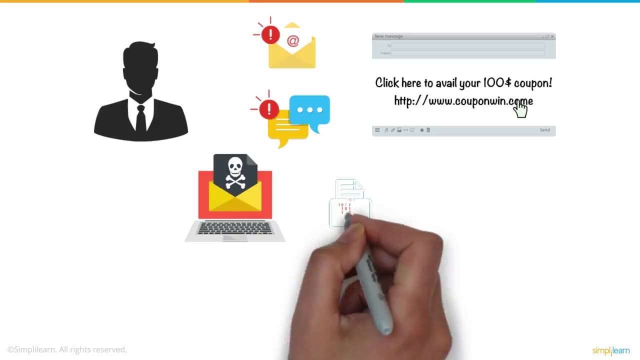 Users tend to click on unknown links received via emails and chat applications, promising rewards of some nature. Once clicked, a ransomware file is installed on the system that encrypts all the files or blocks access to computer functions. They can also be spread via malware transmitted via untrusted application installation or 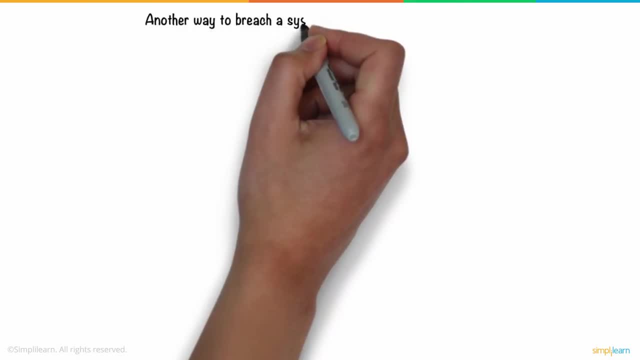 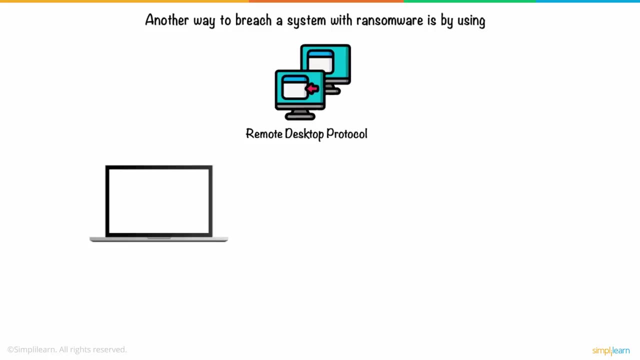 even a compromised wireless network. Another way to breach a system with ransomware is by using the Remote Desktop Protocol or RDP access. A computer can be accessed remotely using this protocol, allowing a hacker to install malicious software on the system. The system can also be used to hack a system with the owner unaware of these developments. 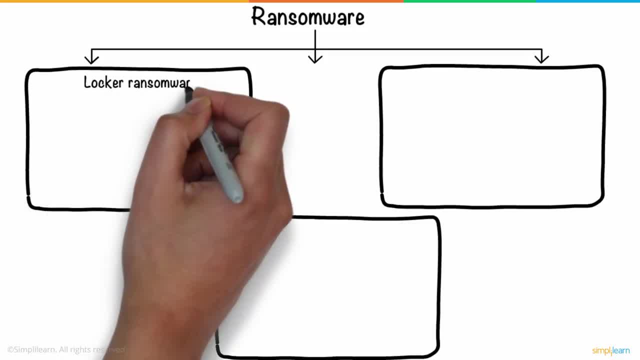 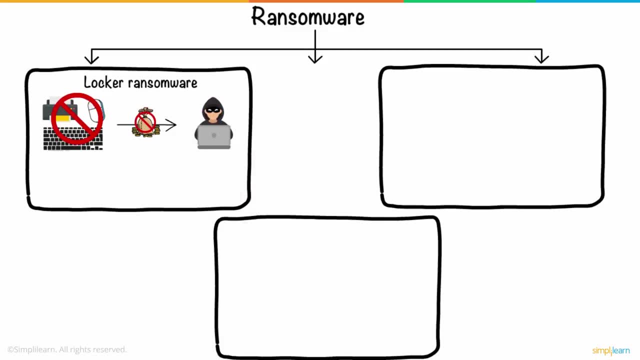 Coming to the different types of ransomware. first we have Locker Ransomware, which is a type of malware that blocks standard computer functions from being accessed until the payment to the hackers is complete. It shows a lock screen that doesn't allow the victim to use the computer for even basic 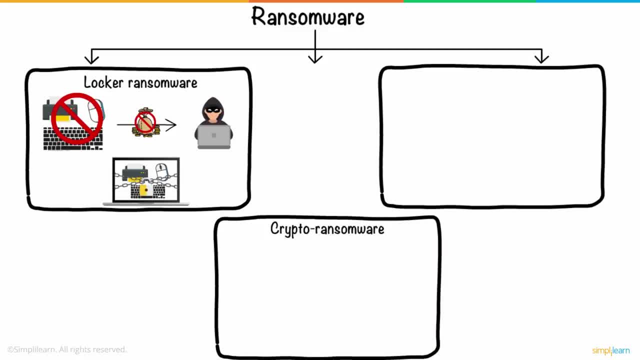 purposes. Another type is Crypto Ransomware, which encrypts the local files and documents in the computers. Once the files are encrypted, finding the decryption code can be done. Crypto Ransomware can be used to encrypt files and documents in the computers. 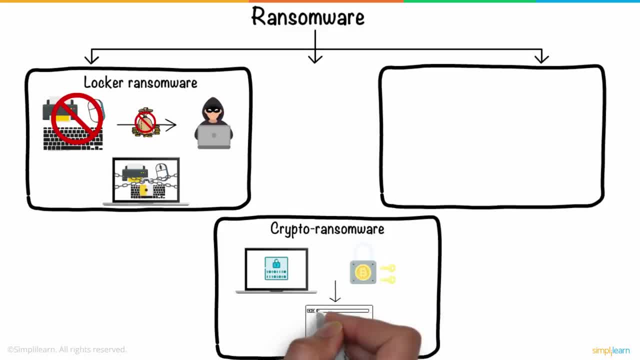 Finding the decryption key is impossible unless the ransomware variant is old and the keys are already available on the internet. ScareWare is fake software that claims to have detected a virus or other issue on your computer and directs you to pay to resolve the problem. 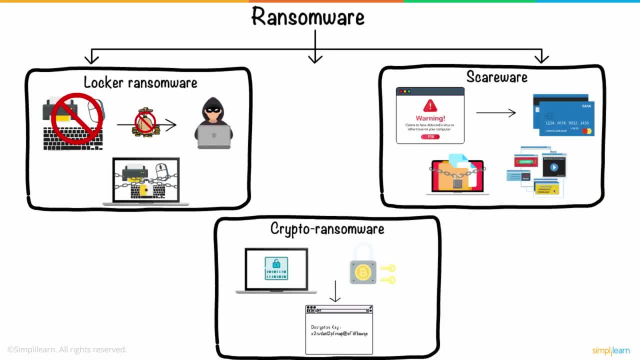 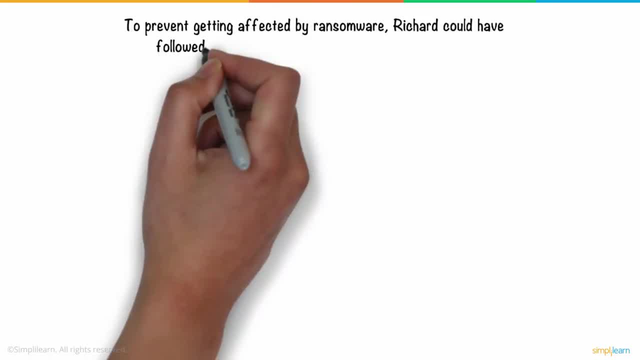 Some types of ScareWare lock the computer, while others simply flood the screen with pop-up alerts without actually damaging files. To prevent getting affected by ransomware, Richard could have followed a few steps to further enhance his security. One must always have backups of their data. 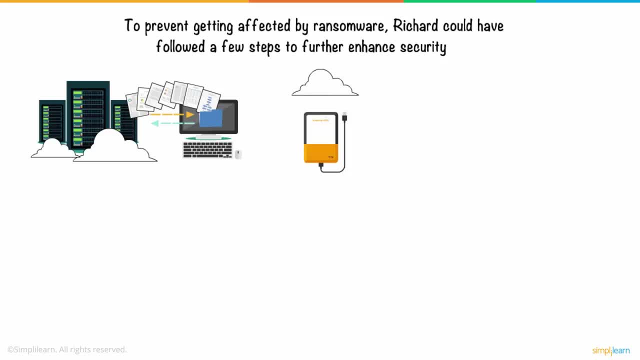 Cloud storage for backup is easy, but a physical backup in a hard drive is always recommended. Keeping the system updated with the latest security patches is always a good idea. Apart from system updates, one must always have reputed antivirus software installed. Many antivirus software, like Kaspersky and Bitdefender, have anti-ransomware features. 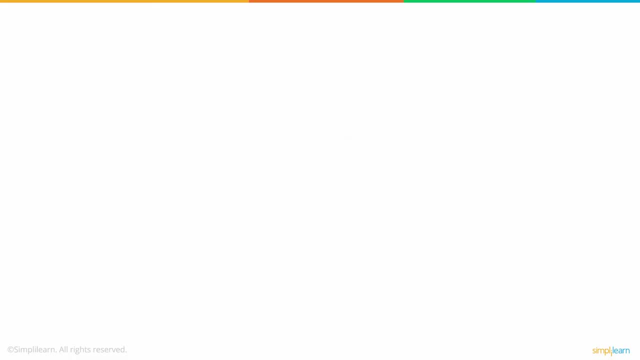 that periodically check for encryption of private documents. When browsing the internet, a user must always check for the locksim on the address bar, which signifies the presence of HTTPS protocol for additional security If a system is infected with ransomware. already there is a website: nomoreransomorg. 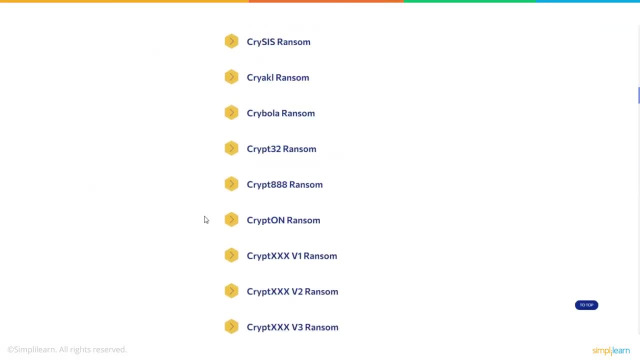 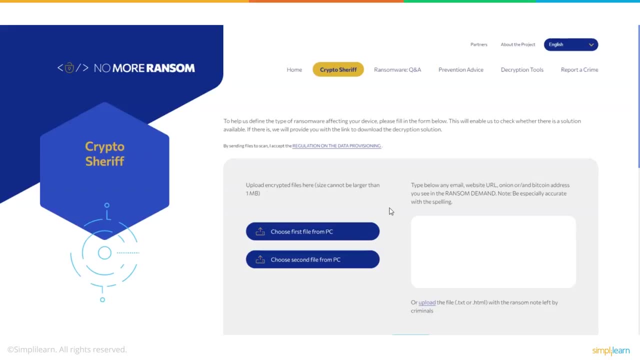 It has a collection of decryption tools for most well-known ransomware packages. It can also help decrypt specific encrypted files if the list of anti-ransomware tools didn't help the victim. So here is a question for you: What is ransomware? 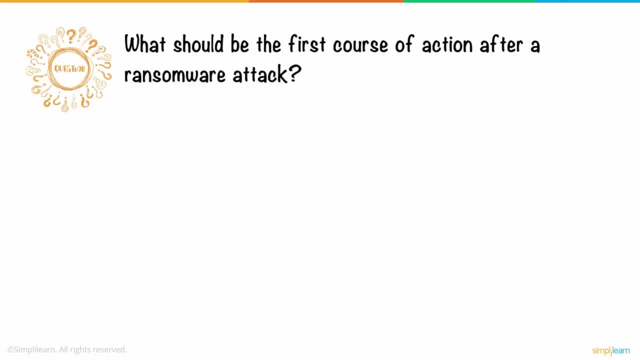 What should be the first course of action after a ransomware attack? 1. Contact the criminal authorities. 2. Run antivirus scan for the entire system. 3. Recover from local or cloud backups. 4. Isolate device from the parent network. Think about it and leave your answers in the comment section, and three lucky winners will. 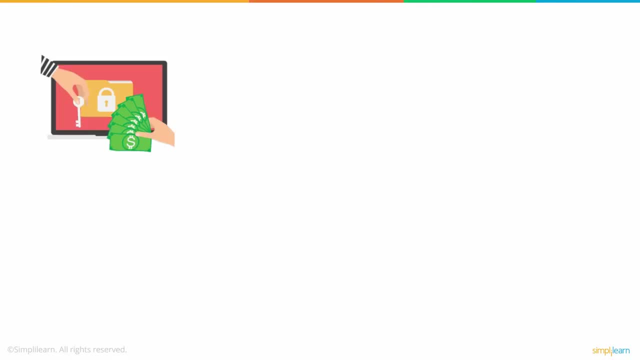 receive Amazon gift vouchers. Ransomware attacks have become increasingly common due to the shift in crime rate. Ransomware attacks have become increasingly common due to the shift in corporate work culture from in-office to work from home. In March 2021, a Chicago-based company called CNA Financial was attacked by ransomware that